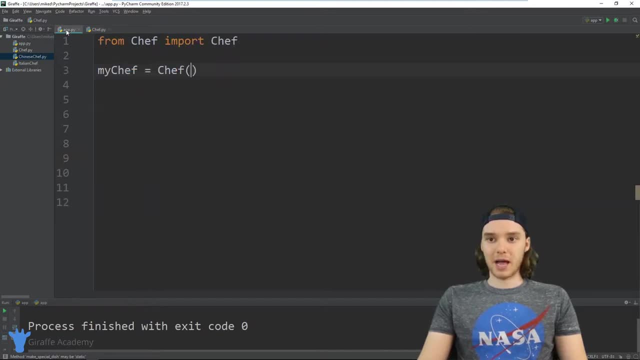 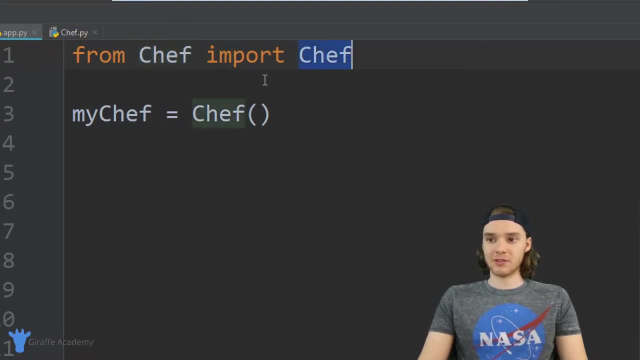 saying whatever the chef is doing. so if I was to come over here to my app dot python file, you notice that I'm importing the chef, so I'm basically allowed to use this chef class now and I can say: my chef is equal to chef. so I'm creating a new chef. 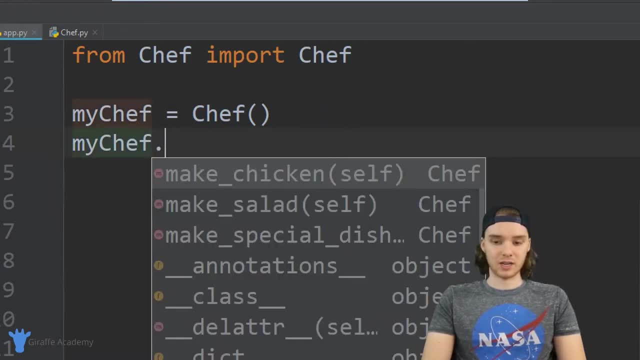 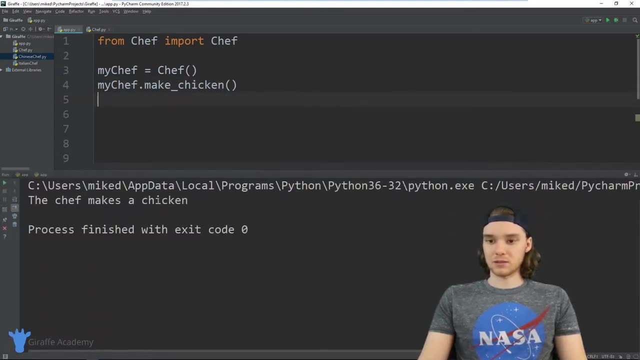 so now, if I came down here and I said my chef dot make chicken when I run my program, now it's going to say the chef makes a chicken. if I said make special dish and I run the program, now it's going to say the chef makes barbecue ribs or because that's the chef's. 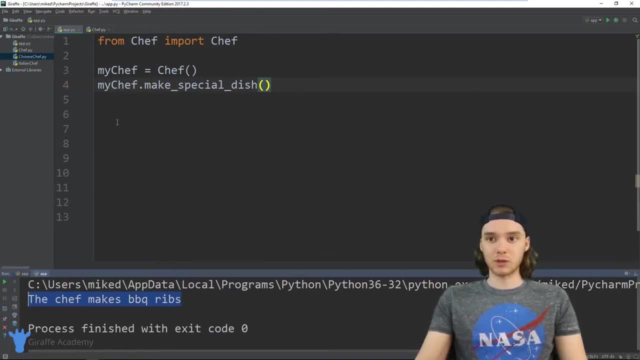 special dish. so I have this really awesome chef class and it works really well. but let's say that I wanted to create another class to model another type of a chef right. so this chef class is just modeling, like some generic chef right, we're representing some generic chef. 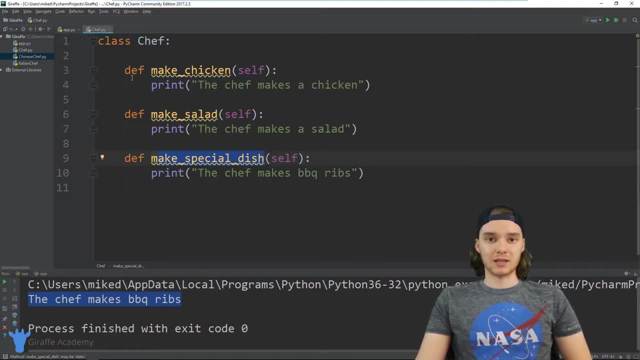 in our program. but let's say that I wanted to create a class that model the different type of chef. for example, let's say we wanted to create a class that modeled a chinese chef. so instead of just a normal chef, this is a chinese chef. well, I actually created a file over here called 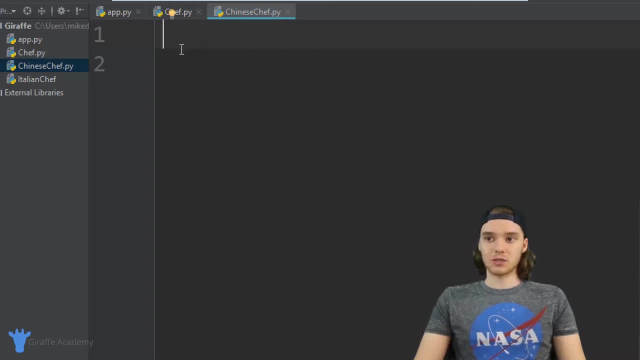 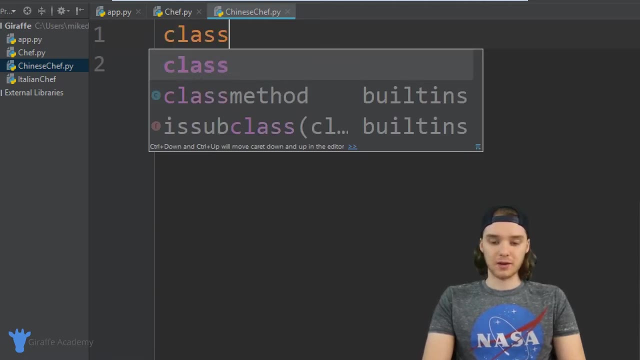 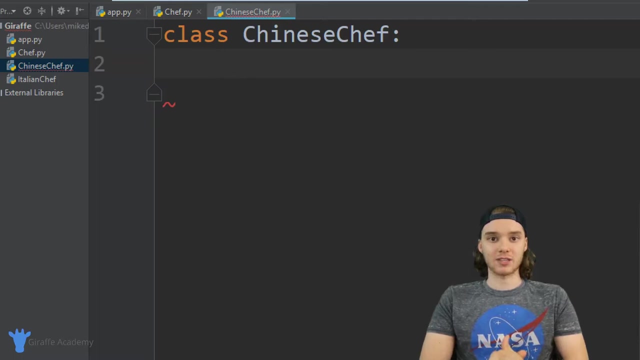 chinese chef dot python so we could actually use this chinese chef dot python file to create our chinese chef class. I'm just going to say class and over here I'm just gonna say chinese chef and basically I just can define everything that the chinese chef can do. 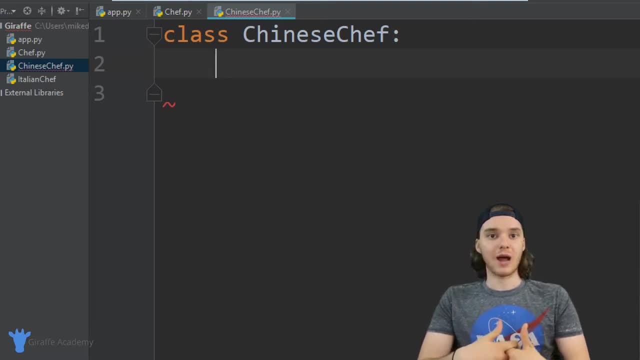 but let's say that our chinese chef can do everything that our generic chef can do. so the chinese chef is like a special chef. right, it's very specific type of chef, but let's say that this chinese chef can do everything that the normal chef can do. so the chinese chef can make chicken. 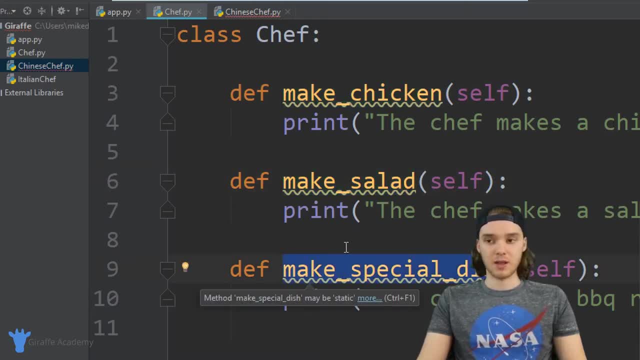 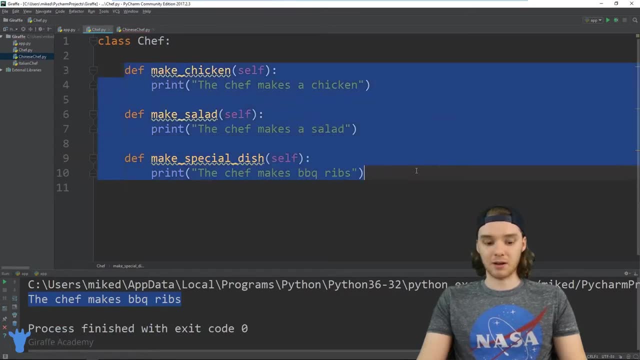 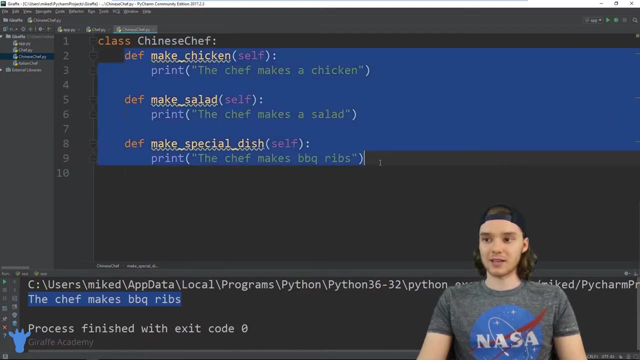 can make salad and can also make a special dish. Well, if I wanted to give this Chinese chef all of that functionality, I could just come over here and I could copy all of these functions And I can paste them in here. So now the Chinese chef can do everything that the other chef can do. But let's say that in addition to all of these things, the Chinese chef can also make a special dish called fried rice. So I could say death And we could say: make fried rice. 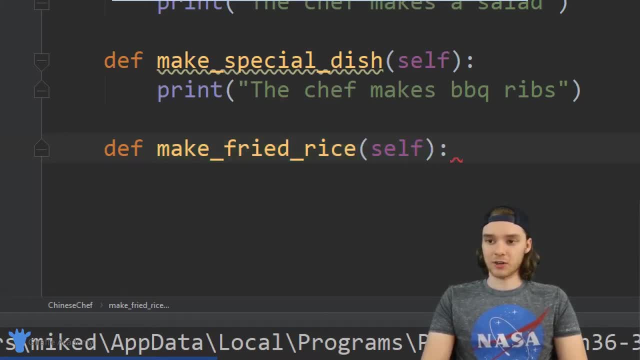 So the Chinese chef has this extra function which allows it to make fried rice. And over here we just say the chef makes fried rice. And let's also say that the Chinese chef has a different special dish. So instead of making barbecue ribs, the Chinese chef makes orange chicken. 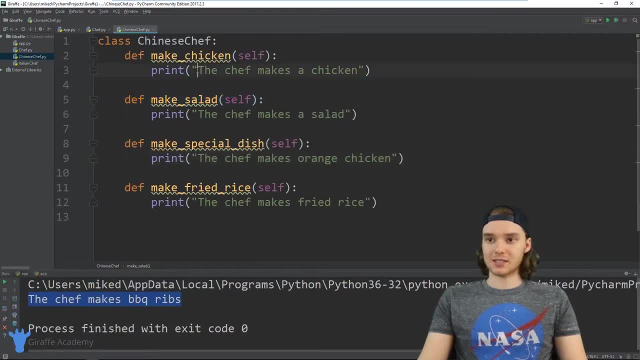 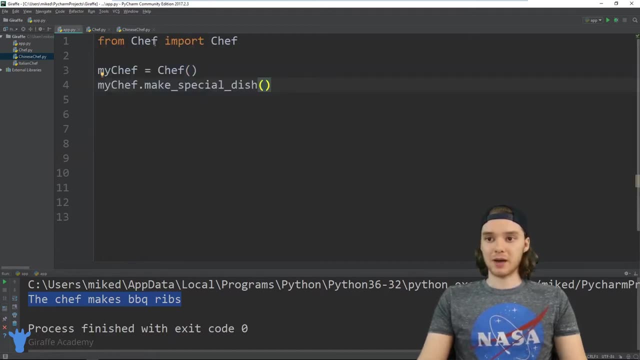 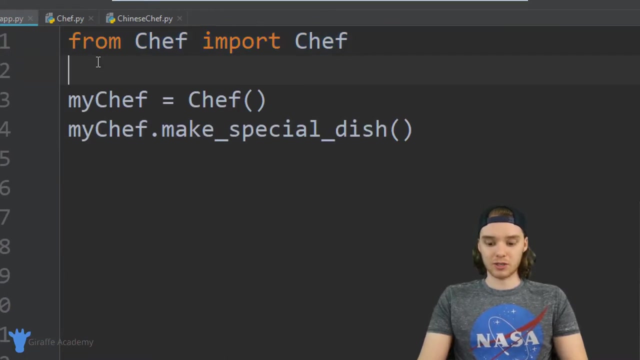 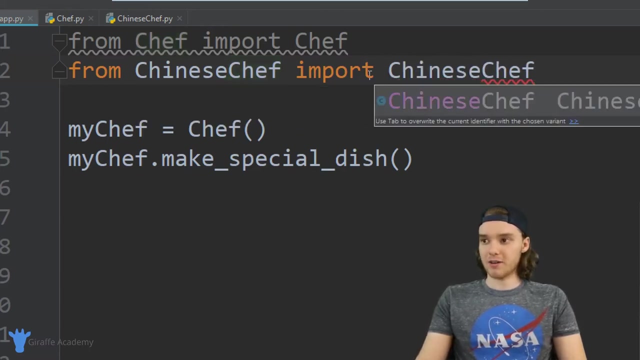 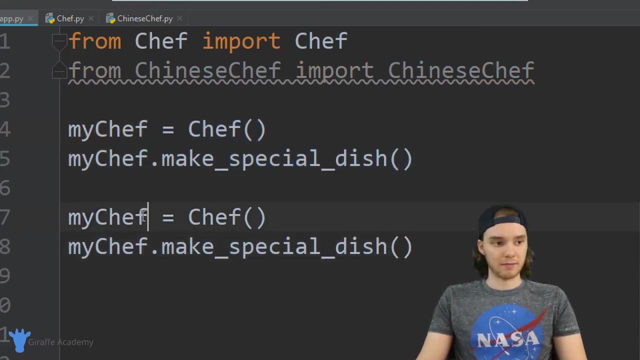 All right. so now we have our Chinese chef class setup And you'll notice that it can do everything that the normal chef could do. So let's go back over to our app dot Python file And I want to create a Chinese chef object. So instead of importing from chef, we're going to just import it from Chinese chef. So I'll say Chinese chef and we're going to import Chinese chef. So let's go ahead and make a Chinese chef object. So down here I'm going to make one and I'll just say my, and then 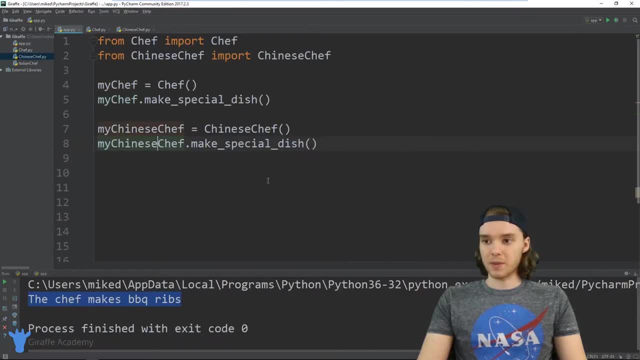 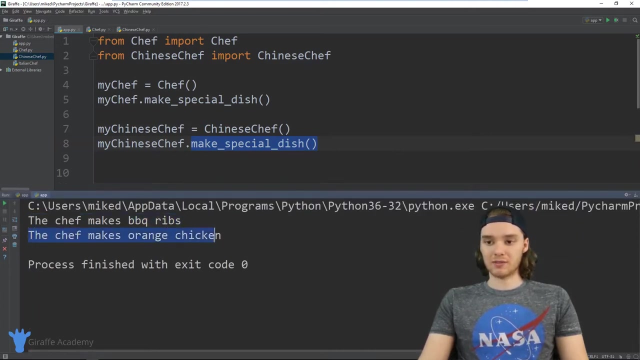 my Chinese chef. we can print out this special dish. So remember, the Chinese chef can do everything that the normal chef can do. So if I say my Chinese chef dot make special dish, when I run this program you'll see the regular chef is making barbecue ribs and the Chinese chef is making orange chicken. So everything works out. And this Chinese chef also has an extra method called make. 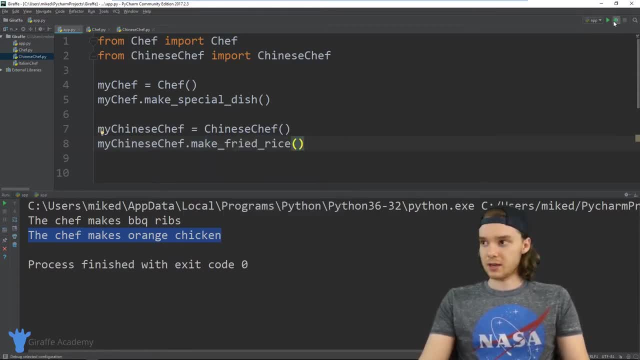 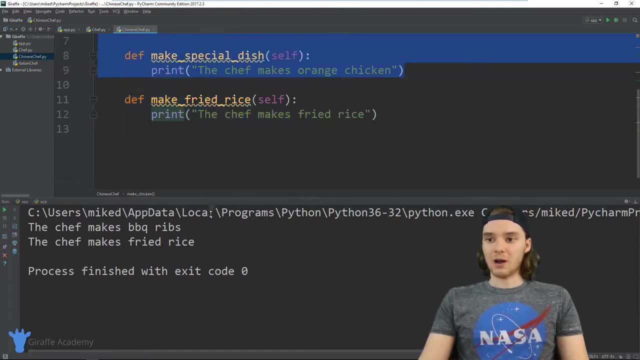 fried rice And you can also make fried rice. But here's the problem: right, When I go over here to this Chinese chef dot pie, I when I wanted to use all of the function, like with rice and Dasik, I have a functionality. 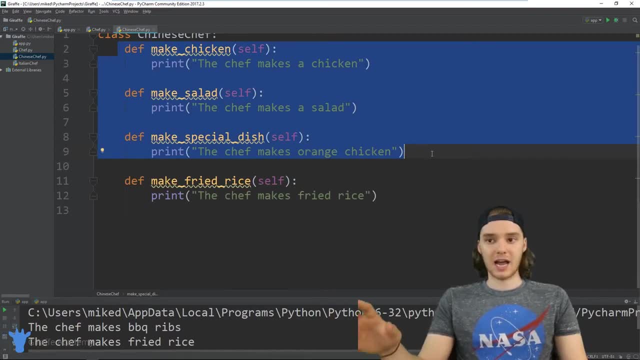 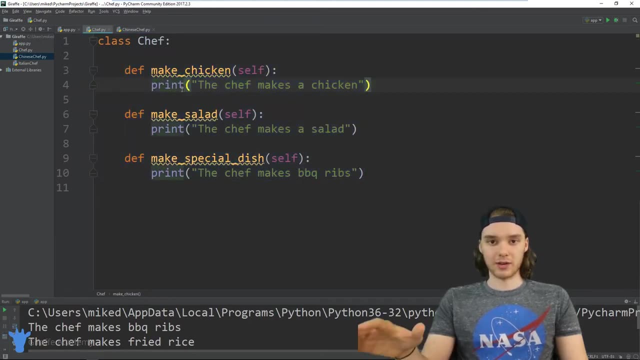 that was inside this chef class. I actually had to copy and physically paste all of these functions down into this file, right, and that's kind of a drag and especially like imagine if this chef had like 20 or 30 of these different functions in it. 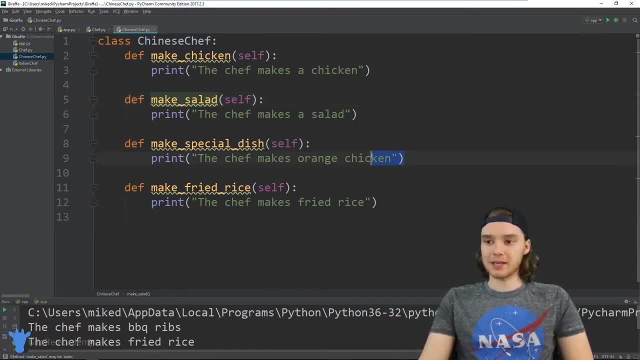 why have to copy- and I have the pace- all of those- anybody inside this Chinese shape, and this is where we can use something called inheritance. so, instead of having account stuff from that chef class, and in order to do that, I can actually just get rid of all of these. 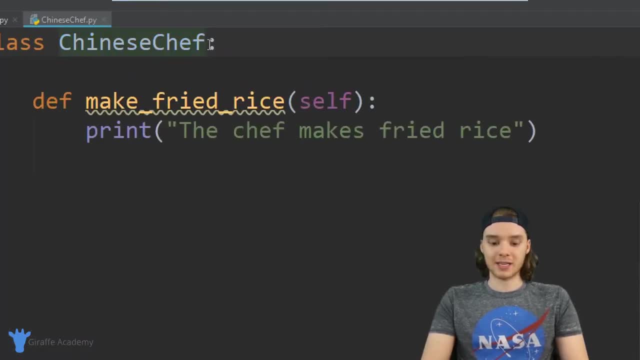 and I can come over here and right next to where I'm saying class Chinese chef. inside of parentheses I can say the name of the class that I want to inherit from. so I can just say chef, and I'm also going to have to import this. so I'm going to come over here and we'll say: 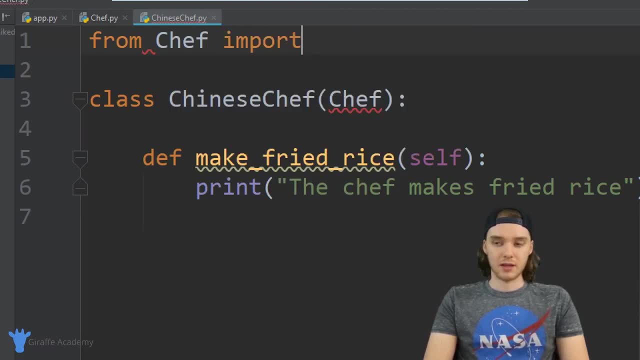 from chef import chef. so basically, what this is saying is: inside of this Chinese chef, I want to be able to use all of the functions that are contained inside of the chef class. so say that one more time: inside of this Chinese chef class, I want to be able to use all of the functions that are inside of this. 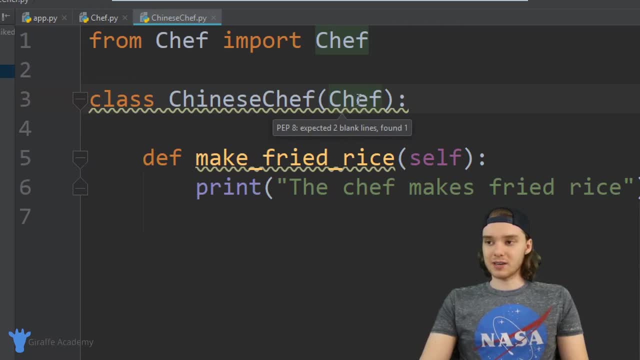 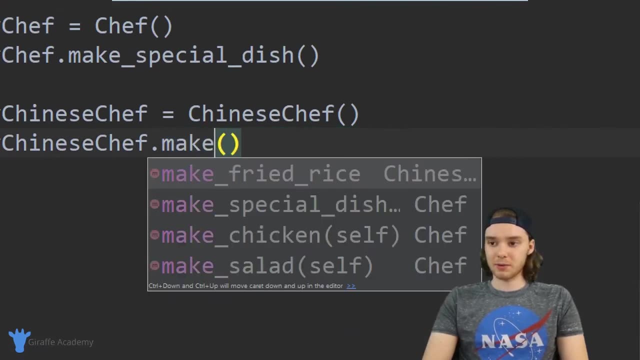 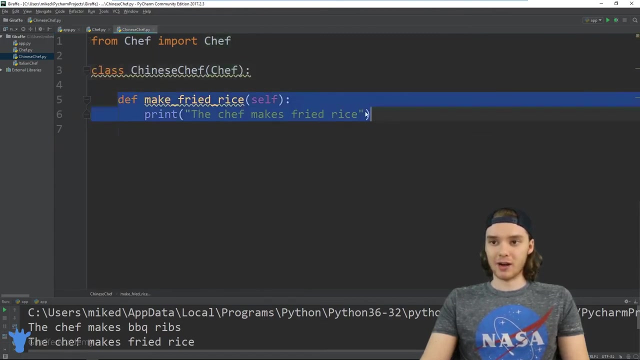 chef class. so by using inheritance here I'm actually able to come over here to this app dot pi file and now I'm still able to execute, for example, like the make chicken function, even though I didn't specify the make chicken function in here, I didn't write it out. 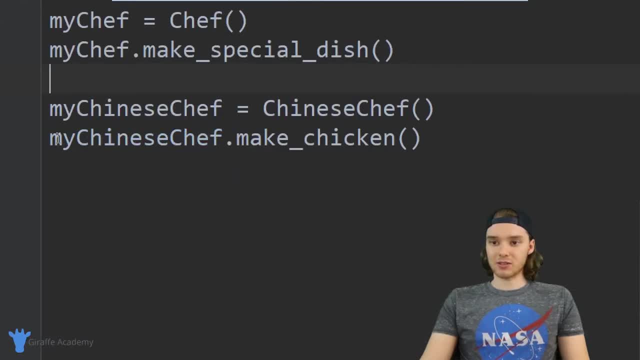 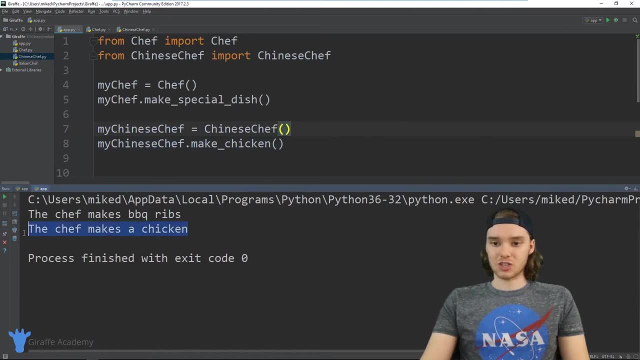 I can still run this program and the Chinese stuff. the Chinese chef will still be able to make chicken. so when I run this program, you see down here it says the chef makes chicken and that's because I inherited the make chicken method from the chef class. but here's one thing that got messed up. 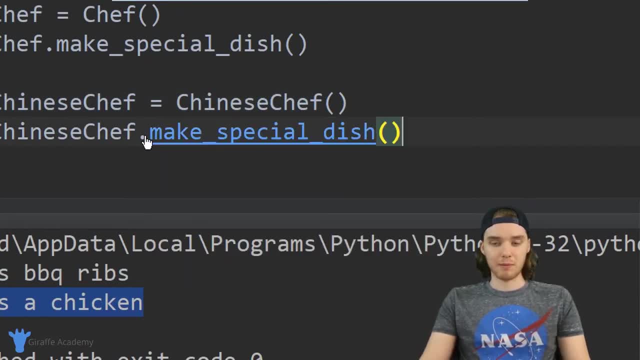 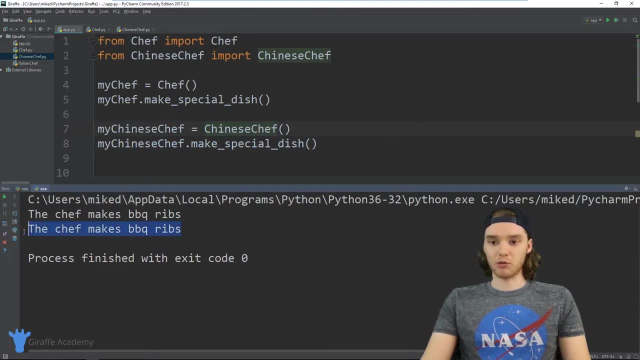 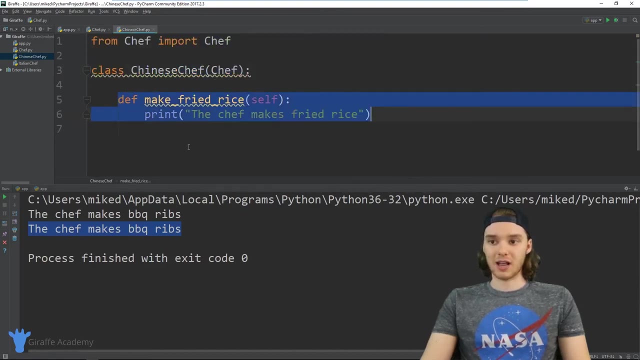 if I come over here and I say: make special day special dish. remember the Chinese chef special dish was supposed to be orange chicken, but now the Chinese chef is going to be making barbecue ribs, because I inherited this make special dish function from this chef class. so what I can actually do is I could come in here and I could. 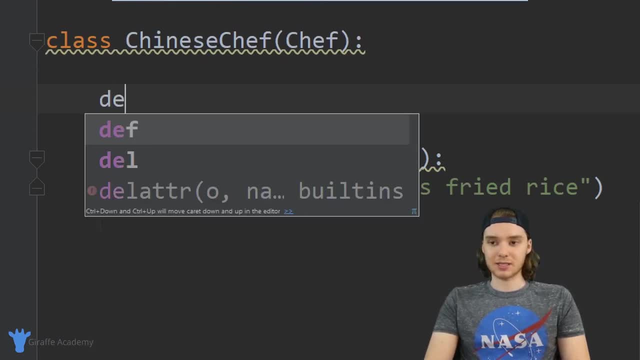 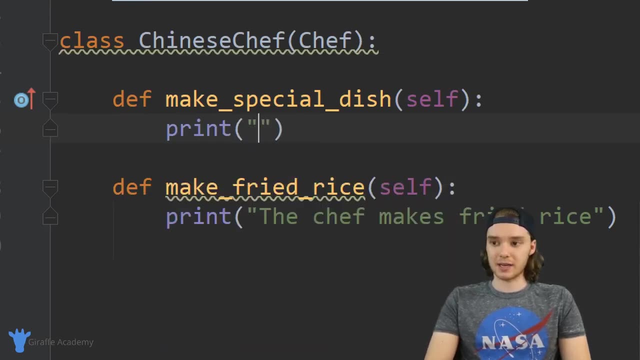 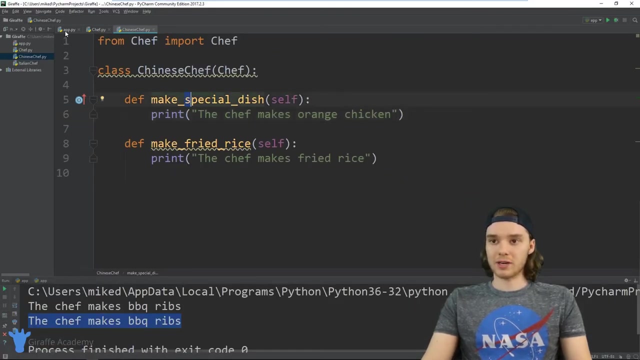 override that, make special dish class. so I could say death, make special dish. and down here I can just override it. so I could say the chef makes orange chicken. and now when I go over here and I run this, make special dish function. now the chef's going to be. 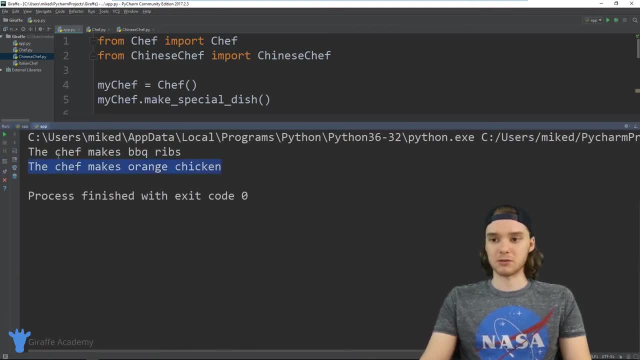 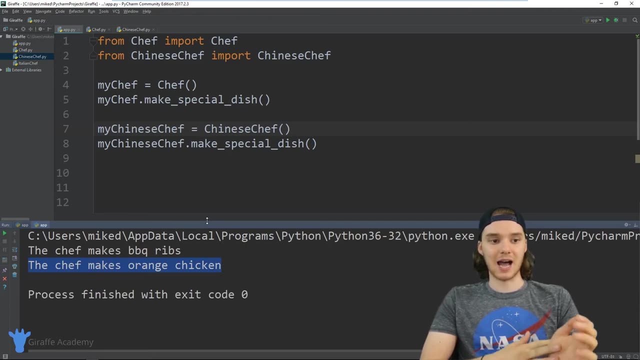 back to making orange chicken, so the chinese chef will make his special dish. so that's basically what inherit- it does in the last video in hair it functionality from an existing class into the new class, and I can actually just inherit all of it without having to write it out. so 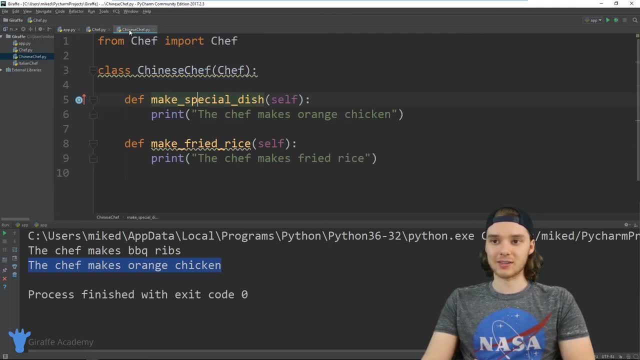 I didn't have to write out make chicken and make salad inside the Chinese class. but the Chinese chef can still make chicken and salad because it inherited that functionality from the chef class. Hey, thanks for watching. If you enjoyed the video, please leave a like and subscribe to Draft Academy to be the first.